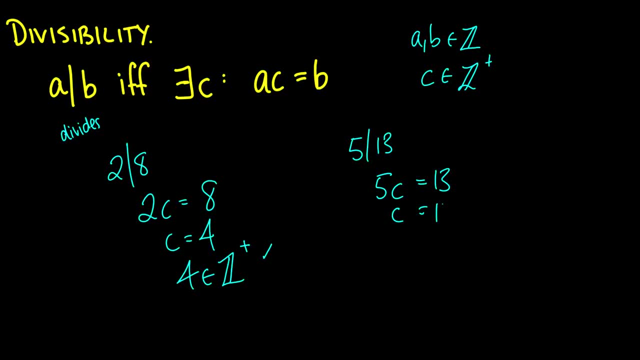 times c is equal to 13,, which means c is equal to 13 over 5,, which I will just rewrite as 2.6, and is that a positive integer? The answer is no. therefore, we know that 5 does not divide 13,. 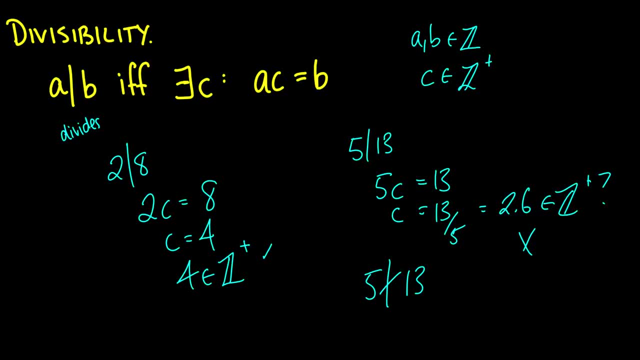 which we just show with a little line through our division sign. So all right, so we're going to start with divisibility. Although it's cool to check out and solve these problems for some number, just to see if there's a nice little piece of division in there, that's not really an important application. What's a? 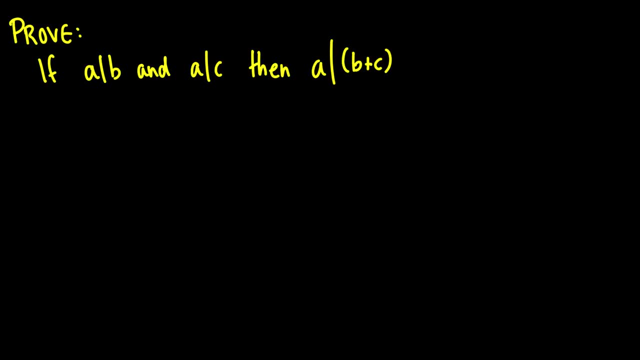 little bit more interesting is proving some theoretical stuff. So I'll do a proof for you and then the next one we'll do together and it'll be fun. So here's the thing: If a divides b and a divides c, then a divides b and c or b plus c. 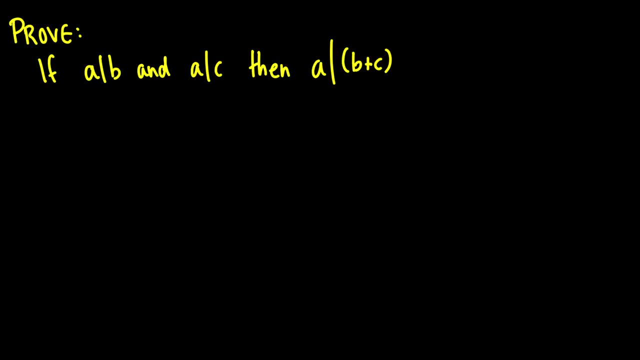 So how do we do this? We're going to do a proof for you, and then we're going to do a proof for you, and then we're going to do a proof like this. Well, we assume the antecedent here, which means: 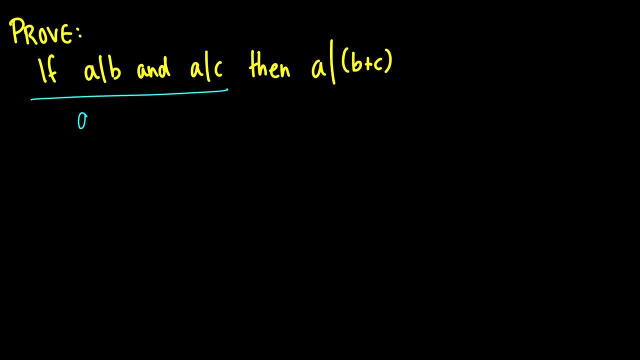 that a divides b. so we know that a times k is equal to b. Again, we don't know what k is, but we know it's a positive integer. and a times j is going to equal c because a divides c. 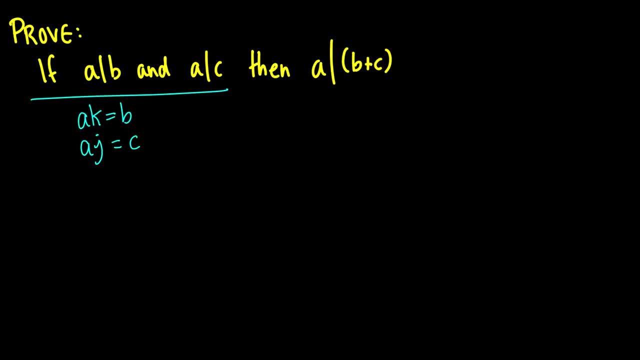 So we want to show that a divides b plus c. So what we do here is we assume b plus c, okay, and this is going to equal. well, we have some equivalences here. so b plus c is going to equal a times k plus a times j. That's good, Now we'll factor. So we're going to factor out the a. 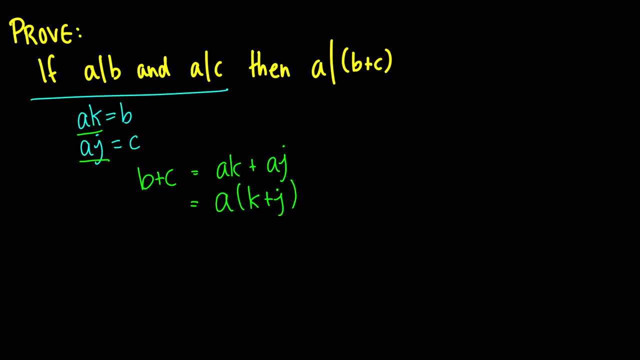 so we'll get a times k plus j. Now to show you exactly how this definition works. I'm going to make some substitutions here. Again, this isn't required, but I'll make them just to prove a point. Really, we're done right here, but what we'll do is we'll 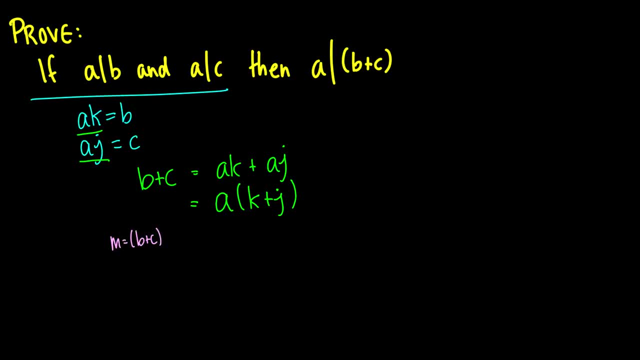 let m equal to b plus c and we're going to let n equal to k plus j. So now we have that m is equal to a times n, which is the same definition of saying that a divides m. but we know that m is. 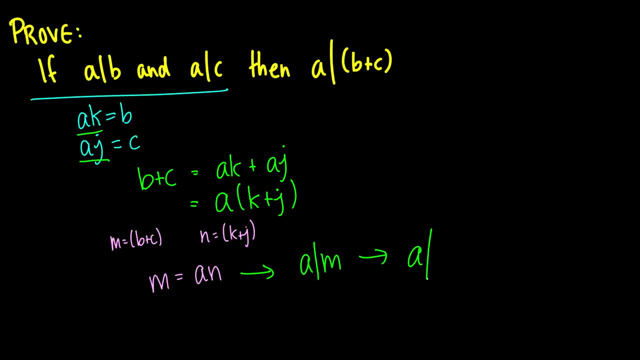 equal to b plus c. Therefore, a is going to divide b plus c. So there's a proof. This is all you really need to do, these proofs, and that's a cool little theoretical thing. So if we know that, say: 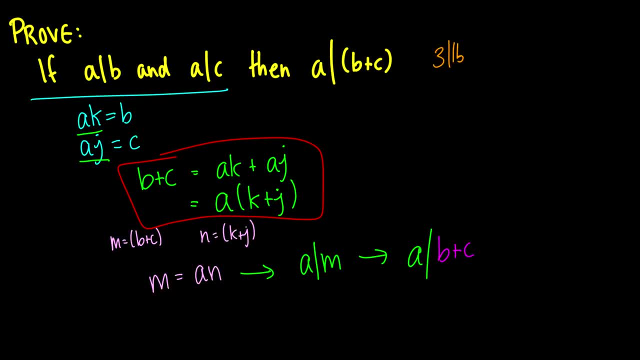 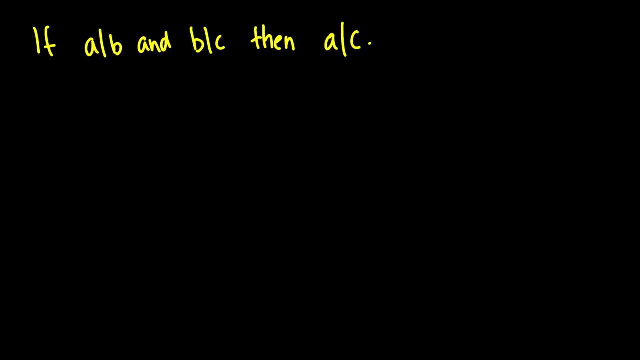 3 divides 15, and 3 divides 9,, then we know that 3 is going to divide 24.. That's pretty cool. Anyway, here's a proof: if a divides b and b divides c, then a divides c. let's see if you can do this. 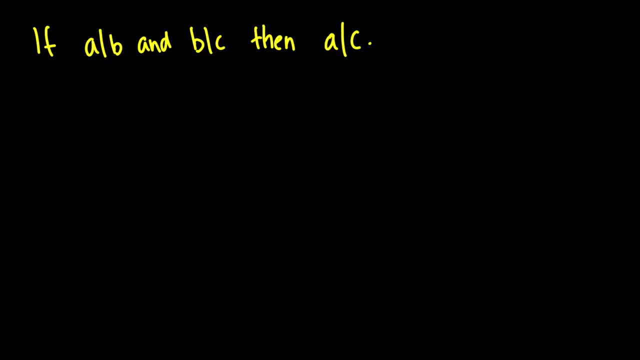 pause the video, try it, and i'll be back in a second. all right, this one's not too bad. we do the same things before. we say, okay, well, a times k is equal to b and b times b times j is equal to c. again we assume this stuff here. so k and j are some positive integer. then we assume c. 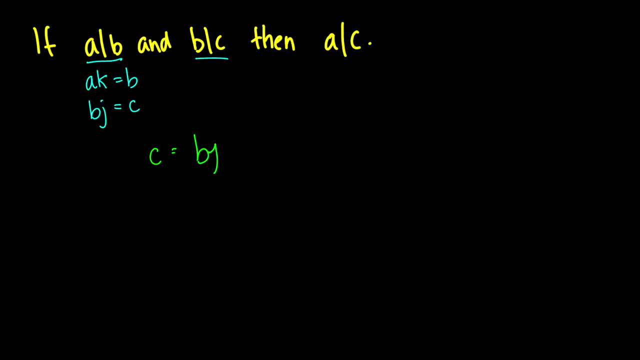 and we know that c is equal to b times j, and let now let's substitute b in there, okay? so now b is equal to a times k, so this is ak times j. now what we'll do is we'll just move the parentheses around so we have a times k times j, and we know this is some number. 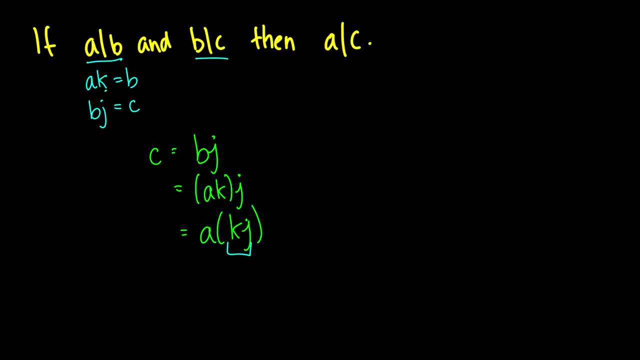 so we'll just move the parentheses around. so we have a times k times j, and we know this is some number. it's some positive integer, because k is a positive integer and j is a positive integer. therefore, when they multiply, they will be a positive integer. so we can conclude from this that a divides c, so 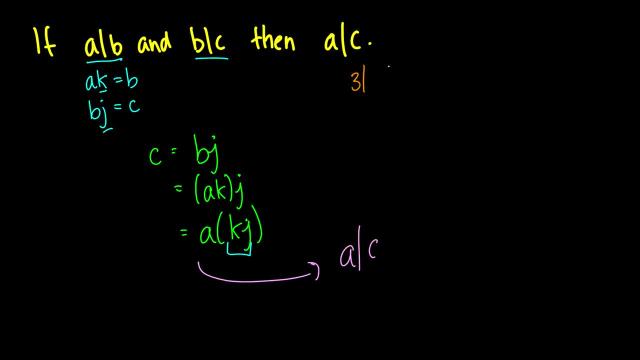 that's pretty cool. for instance, if 3 divides 6 and 6 divides 18, then we have that 3 divides 180. I really hope that 6 times 18 it's. it's been a while. I think that's right it does regardless. so 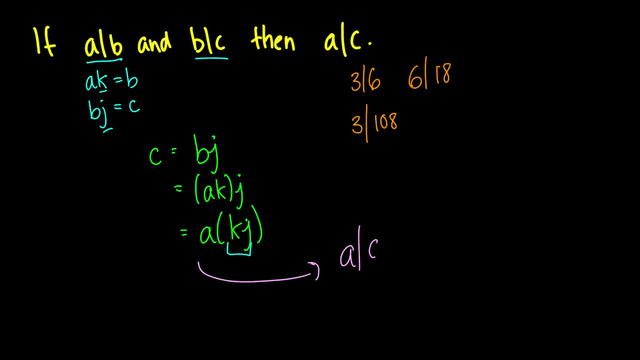 it's all good, but that's two ways and two different proofs you can have. of course there's a lot more proofs. in fact, I really suggest you do a fun one, which is: if a divides C and B divides D, then a B divides CD. in fact that might not be true, so I don't know. you might want to. 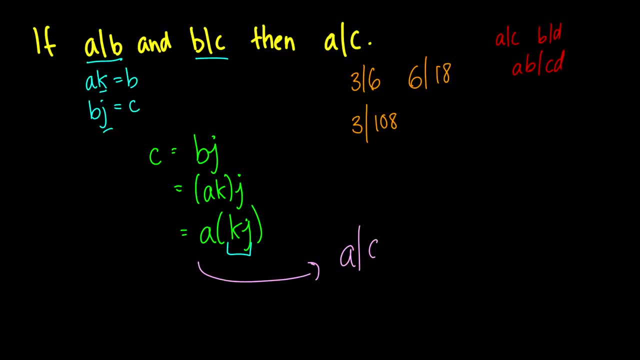 check it out yourself. but I do want to point out one interesting property here and that is here's. I'll draw a little thing here: this is a, this is B, this is C. we have some nice relation arrows here: a divides B, B divides C. then we find out: 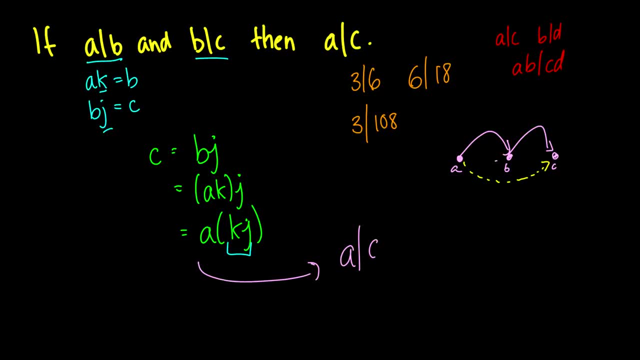 that we get a nice little transitive line here. so this division is transitive, now a a division is transitive now a non-transitive division is transitive, now a non-transitive division. another interesting property of division which I just want to make sure is not there, okay, is that? 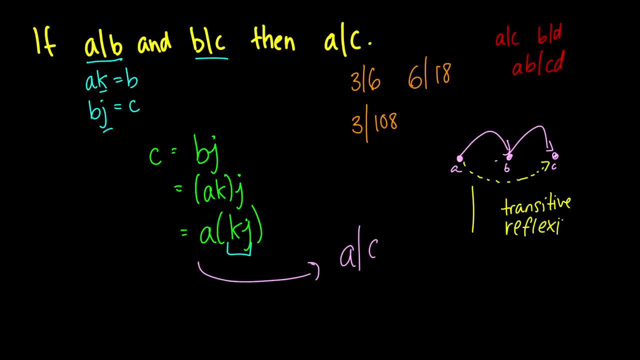 it's also reflexive, since every number is divisible by itself. but is it symmetric? and well, the answer is no. in fact, it's going to be anti symmetric in. it's not okay. it's not necessarily anti symmetric, it's asymmetric because in the case where a divides a, it's. 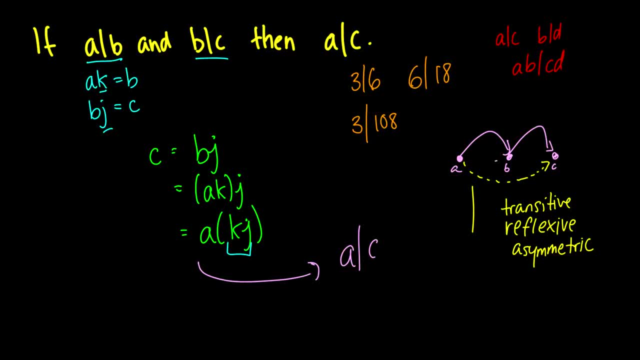 also true that a divides a, but some interesting properties there which you may remember from relations. so do what you wish with that information. perhaps something like this may come up on a test: it's always fun to take information from two different sections and, on an exam, ask a question about how they relate. 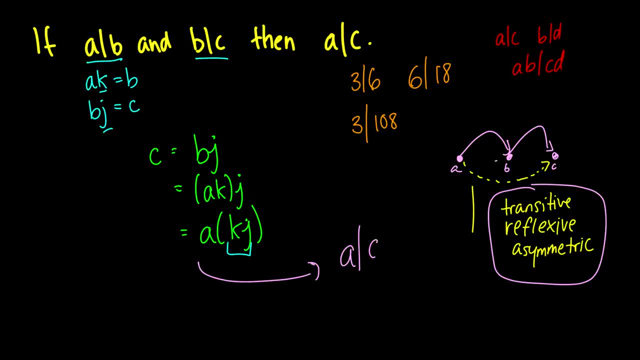 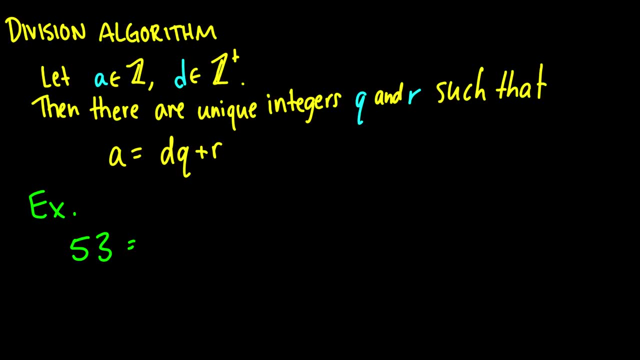 to each other. it's pretty cool, but those are some basic division proofs. now we're going to move into the division proofs. now we're going to move into the division proofs. now we're going to move into the division algorithm and what we say is: okay, let a be an integer and D be a. 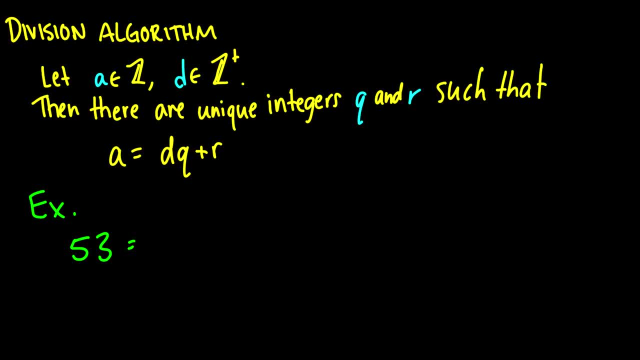 positive integer, then there are unique integers Q and R, such that a is equal to DQ plus R. so basically, this means is: any number has some divisor plus a remainder, and you can break it up like this: now, this is important for a later algorithm, so I'm going to demonstrate this in this video and then when we get